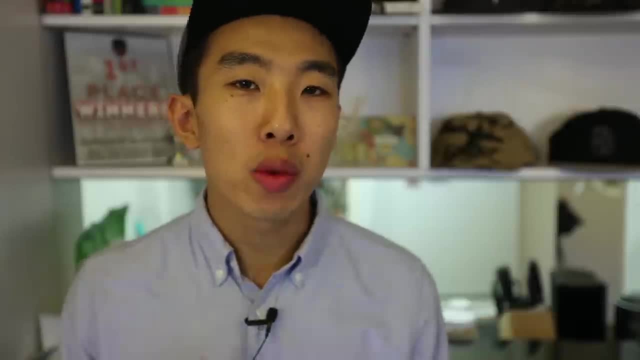 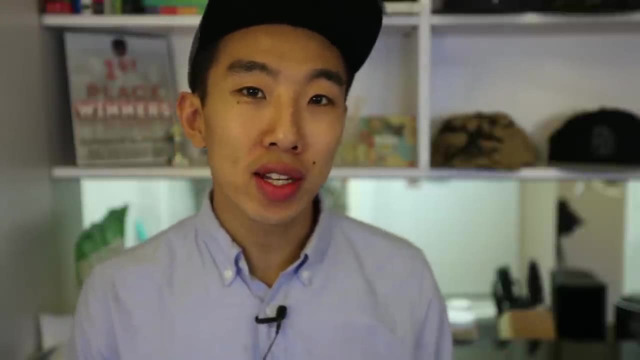 or how could they remember my 10 favorite drinks? Let's just think about how would we design a system like that. How would you design a system like that? Lucky for us, Starbucks has already solved this problem, and the way they solved it is exactly how Sessions and Cookies work on the internet. So 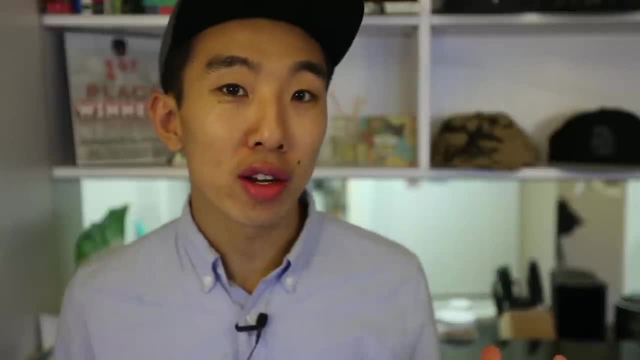 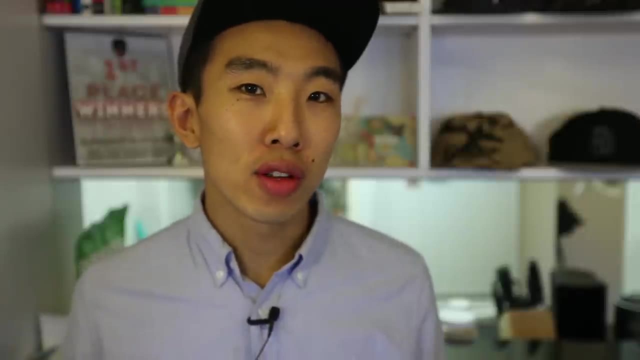 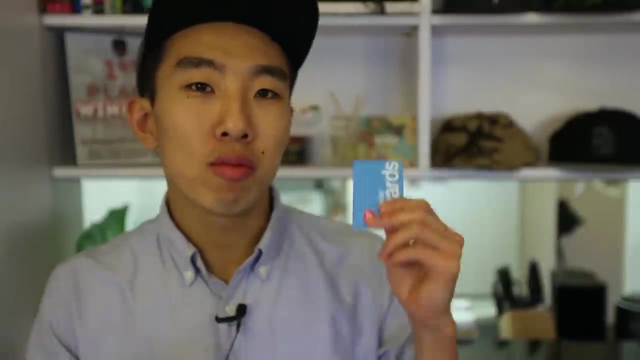 the way they've solved it is: they give you a Starbucks card that you carry with you, and what that Starbucks card actually does is give you a very stateful interaction with Starbucks, and we're going to talk through that. So what exactly is a Starbucks card? anyways, This is not a real 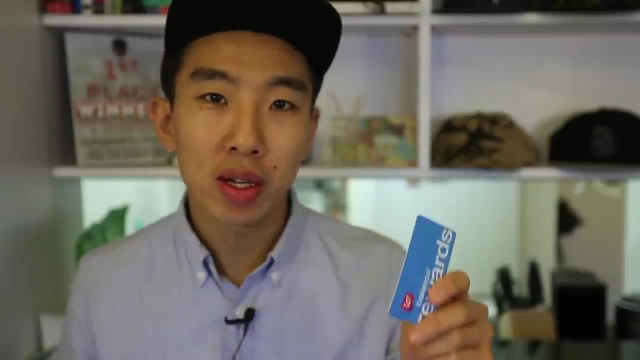 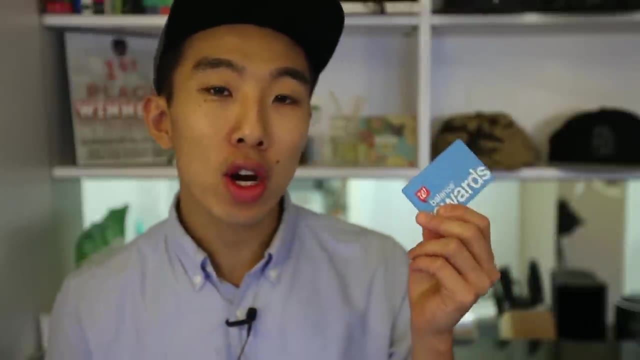 Starbucks card. It's a Starbucks card that you can carry with you. It's a Starbucks card that you can carry with you. It's just a card that I have. But what does this really mean? This thing right here actually means two different things. right, When you carry this card around, this is your. 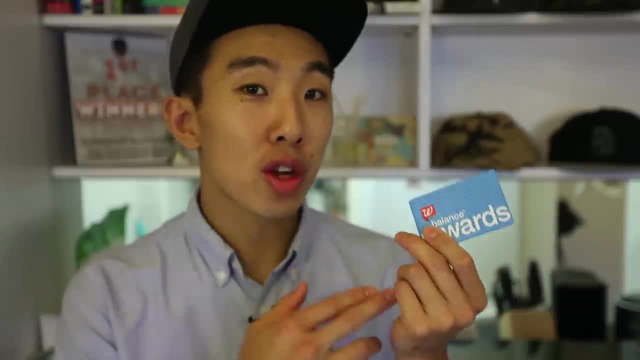 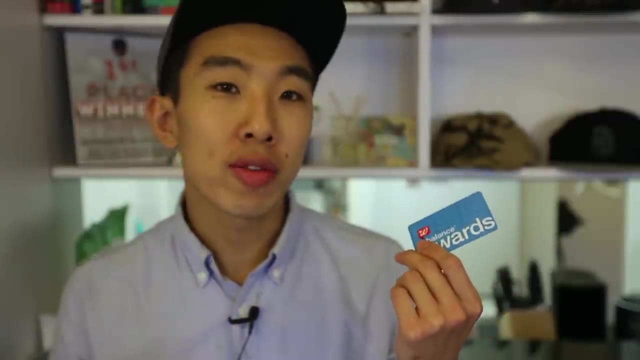 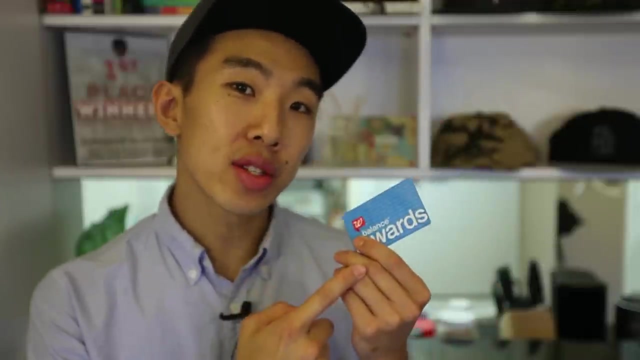 identification for Starbucks: right, But for Starbucks, they've already made an account for you to track all your stuff. Like the last drink you ordered your top 10 favorite chocolate drinks. two parts, right, This is what you carry around your identification, but it matches. 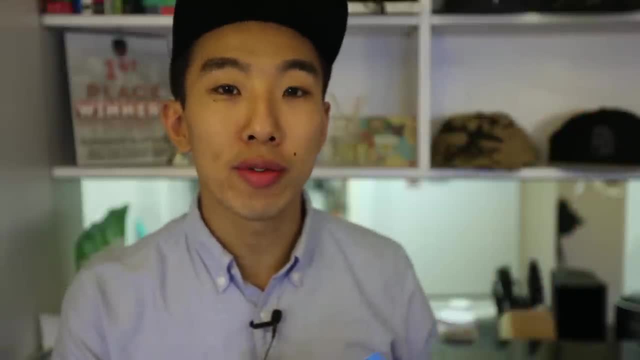 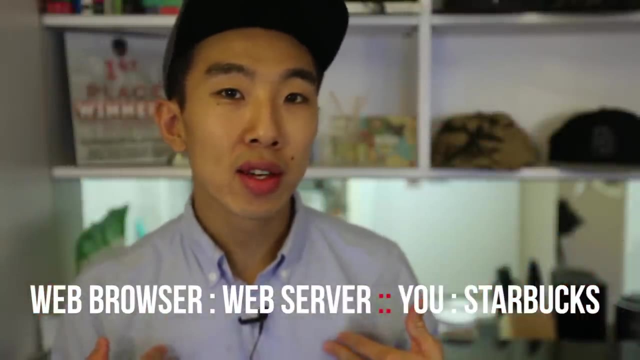 a thing on the Starbucks server where they're tracking all your info. So for this whole example, this whole example is kind of just analogous to the internet, right? I'm actually the client ordering my drinks at Starbucks. I'm like a web browser for the internet and Starbucks. 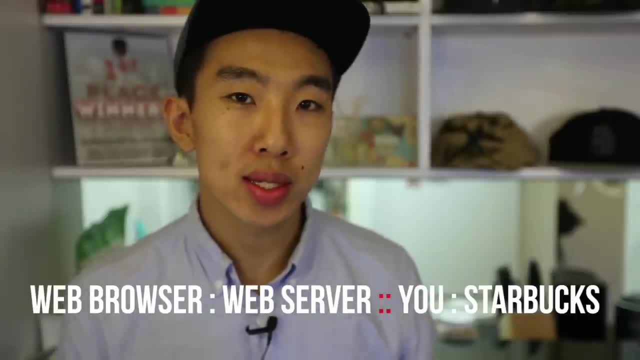 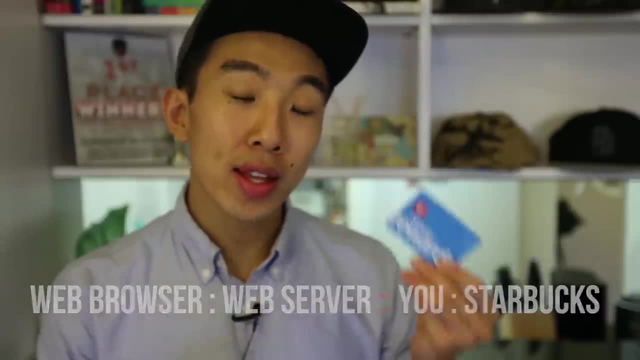 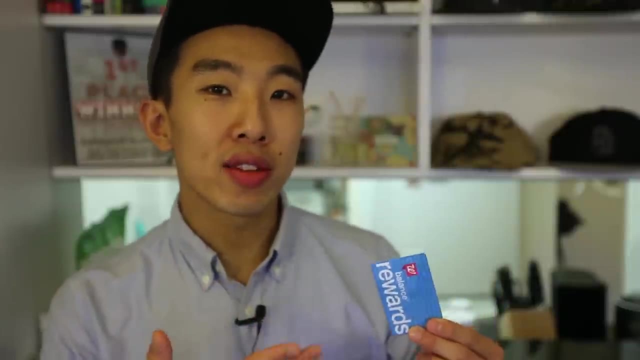 is kind of like a web server servicing my requests. So this ID card, the ID card that you carry with you, this identification that the client always carries, that's called a cookie. So if we have our cookie right, the opposite thing to make this cookie even useful is the session. 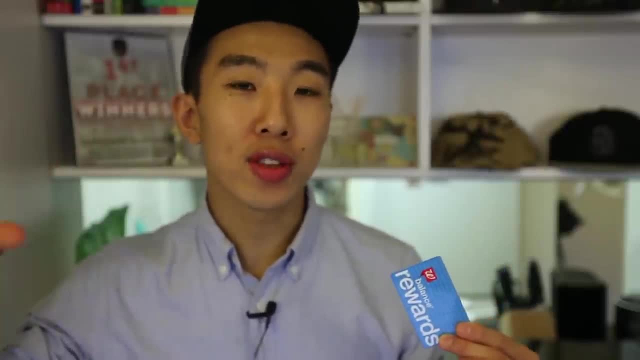 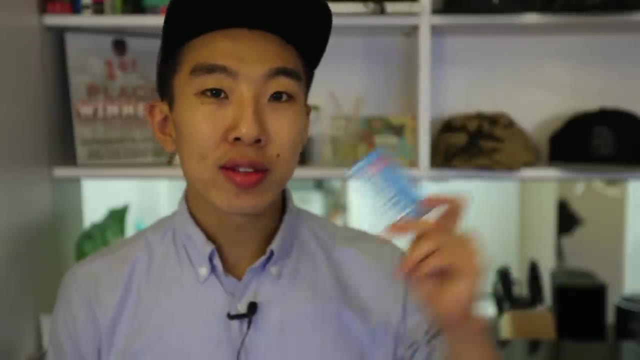 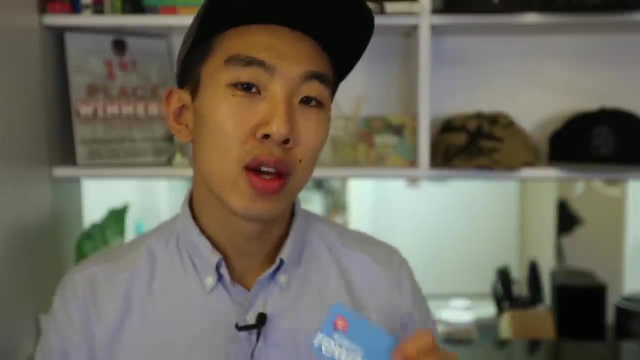 which lives on the server. So Starbucks is tracking a lot of different sessions for all their different coffee drinkers. So why this cookie is important? because it's used to match up with the right session. This is my identification, so Starbucks knows to retrieve my session Hope. 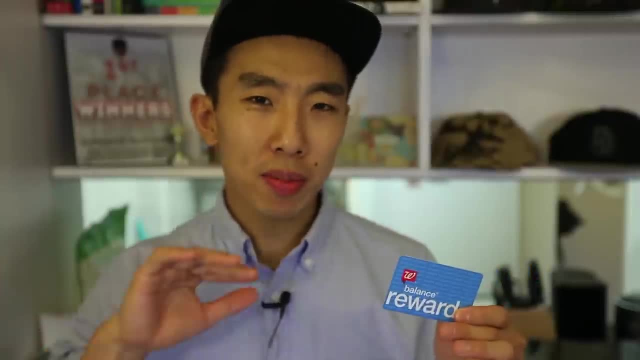 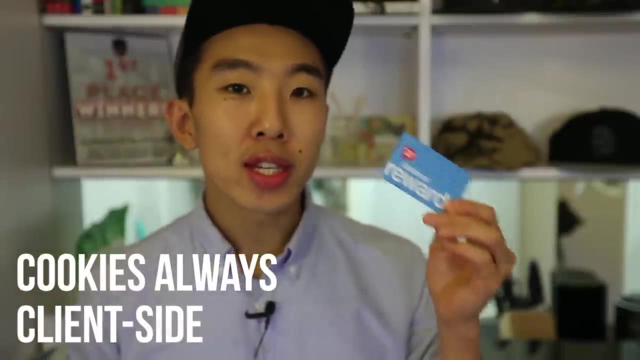 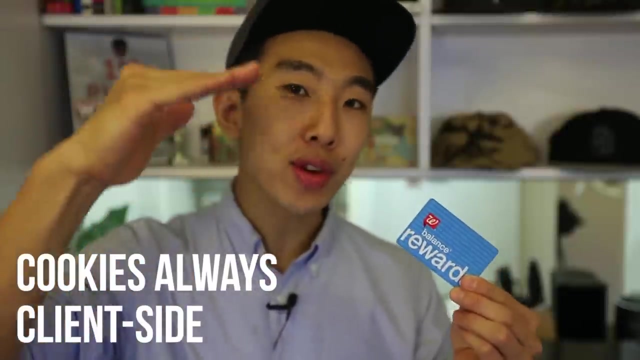 that made sense, All right. just going to repeat myself again to make it extra, extra clear: I'm a client. Starbucks is a server. This identification card or cookie is always client side. If you open up your browser, if you have Chrome developer tools or anything, you can see every single. 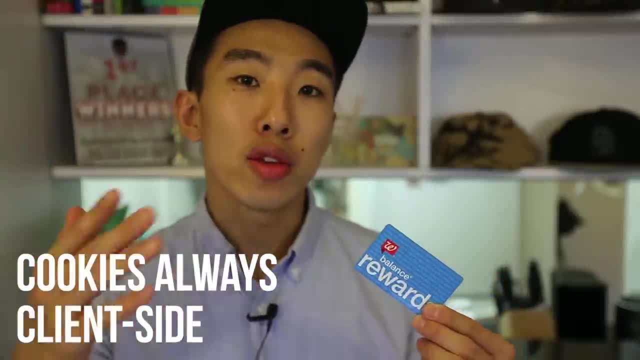 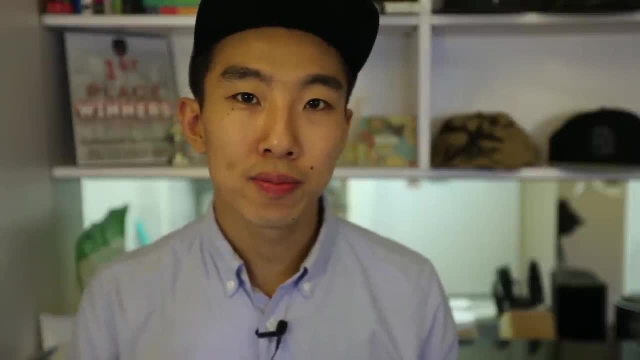 cookie that your browser has saved for all the different websites you've visited. So it's always client side And the session is sometimes, but not always, server side. If I go to Starbucks, I'm going to show them this first right. I'm going to show them my identification so they can get. 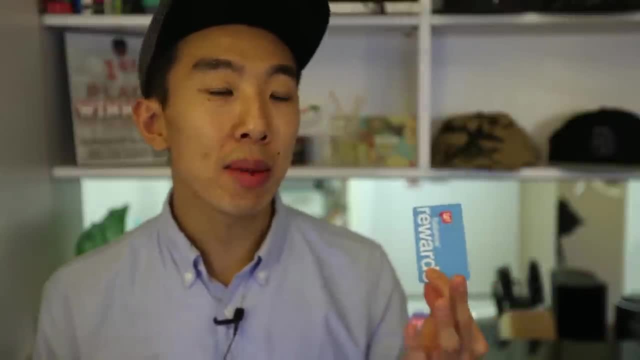 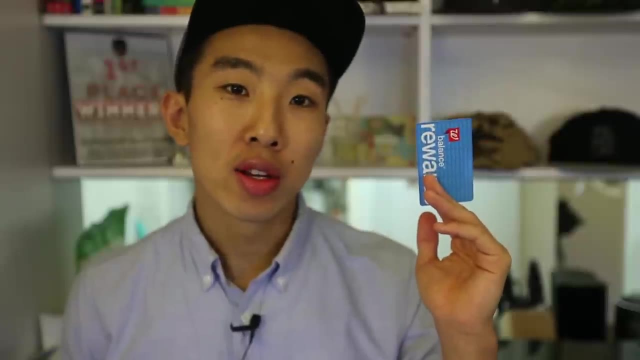 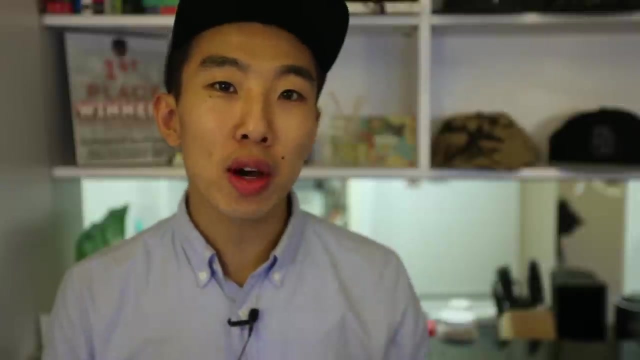 whatever, whatever information they need about me. It's the same thing with web browsers: Every single HTTP request made by your browser sends a cookie along, so the server can do something smart with it. All right, so I hope everyone's slowly digesting this, but you can see how the Starbucks card and Starbucks 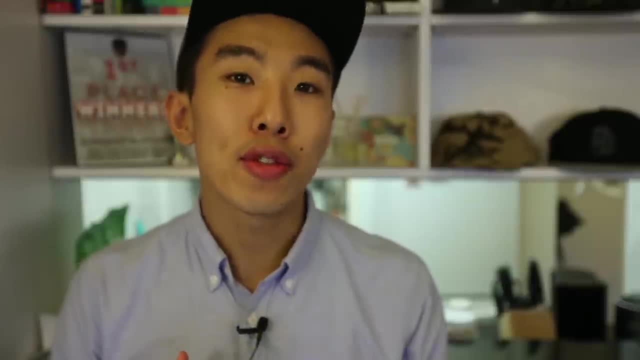 tracking my favorite drinks. that's kind of giving statefulness to my interaction with Starbucks. right At the beginning of the video I told you my interaction was stateless: order a drink on Monday. order a drink on Tuesday, order a drink on Wednesday. But once I have statefulness, 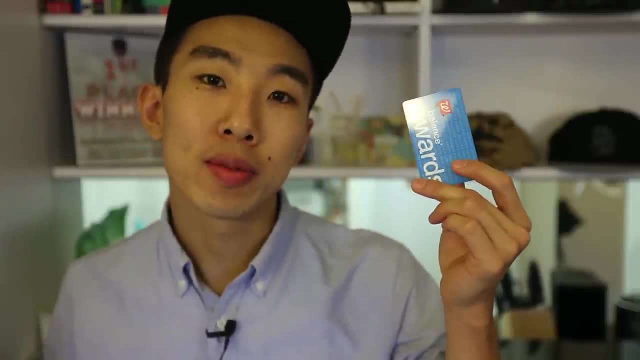 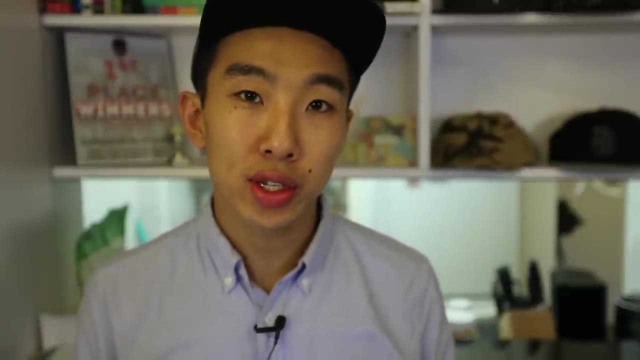 my experience gets much better. Hopefully, This is the most important sentence to understand, And if you understand this sentence now, you understand sessions and cookies. Sessions and cookies are what makes HTTP stateful. I'll just say it one more time to maybe it'll sink in. But remember from: 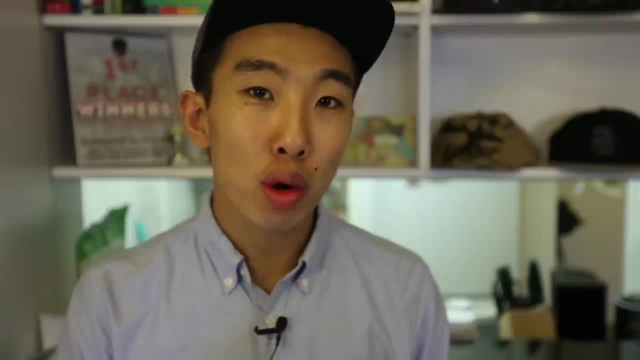 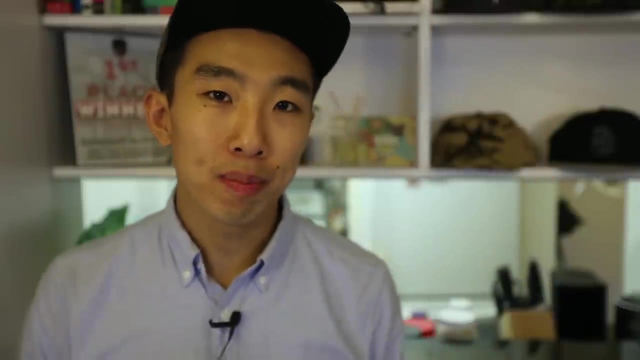 the first video. HTTP is naturally a state list, Protocol sessions and cookies make it stateful. Okay, guys, one last note before we wrap it up. But, as you said, cookies, always client side. remember that when you hear the word cookie. 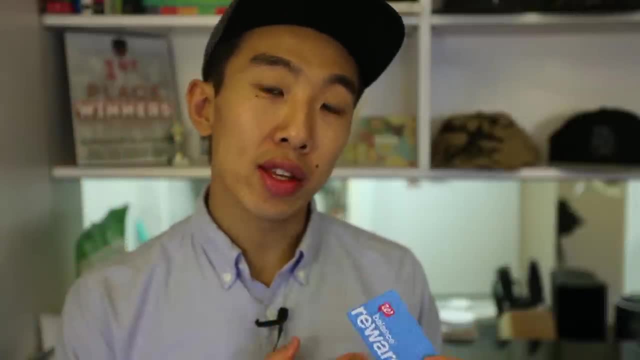 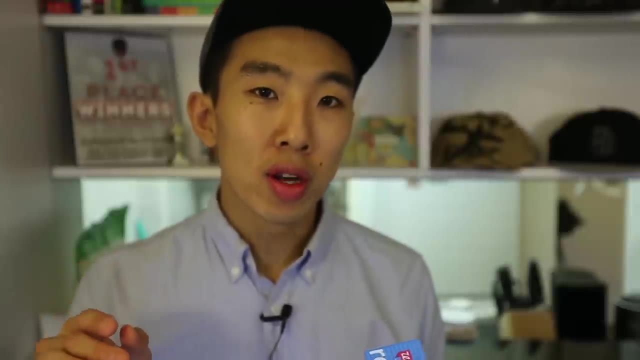 just think client side and the browser is handling your cookies right. But I mentioned earlier that sessions where our sessions stored, normally they're stored on the server, But actually sometimes some applications actually choose to store session information on the client as well. 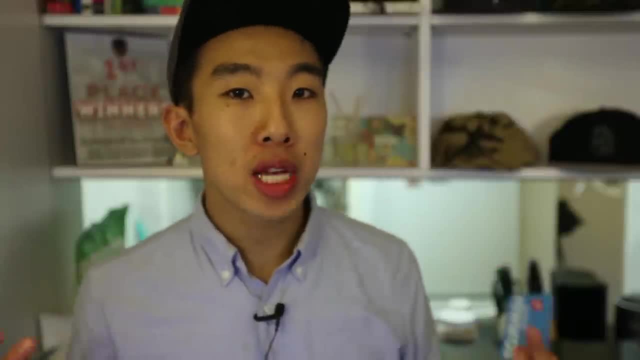 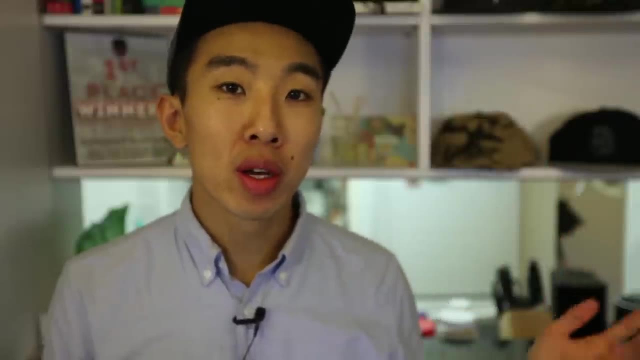 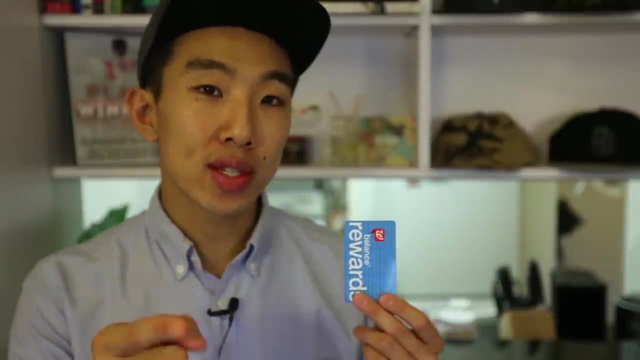 And let's just talk about that real quick. For any web developers out there, I'm sure you know what rails is probably one of the top, if not the most popular web framework in existence, or maybe right now. but by default, if you use the latest rails, they actually store the session on the client by default, And this